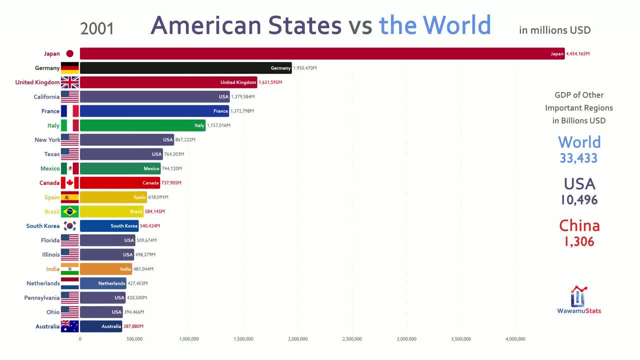 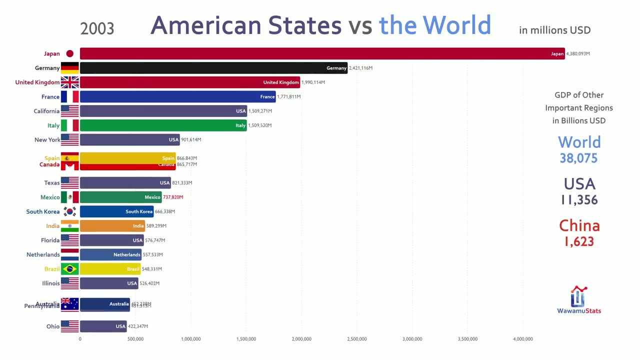 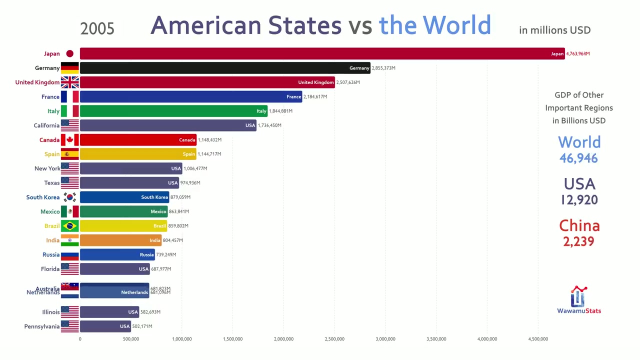 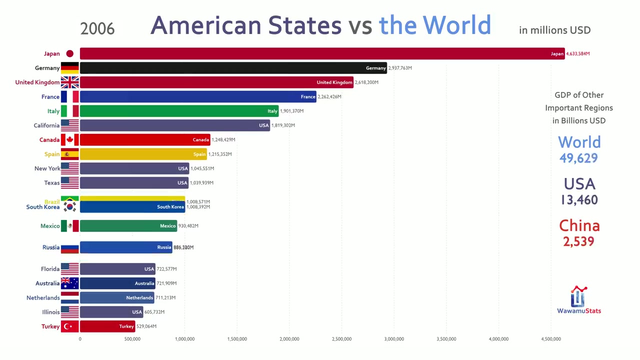 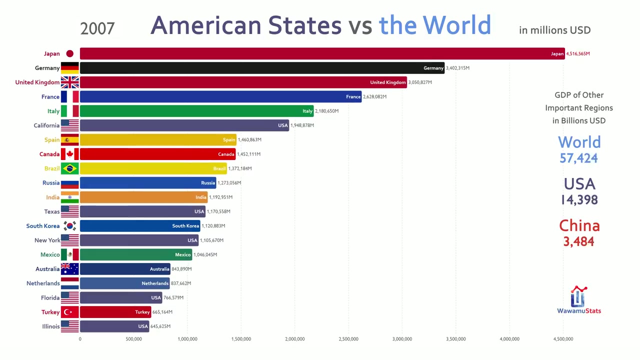 Thank you very much for watching. Thank you very much for watching. Thank you very much for watching. Please subscribe to the channel and press the bell icon to receive notifications when I upload a new video. Thank you very much for watching. We'll be right back. 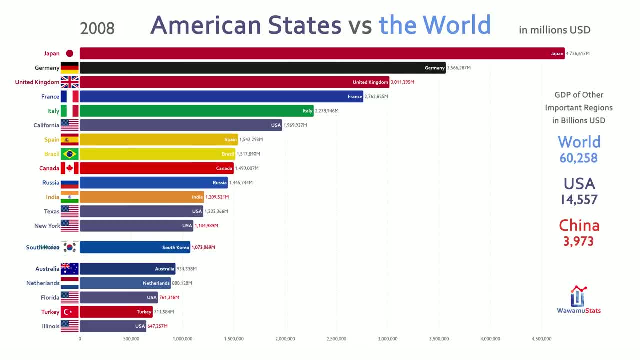 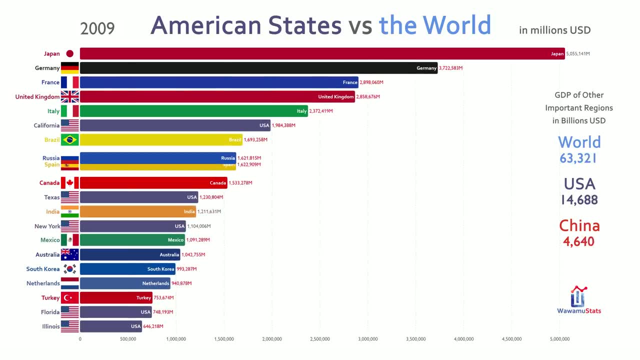 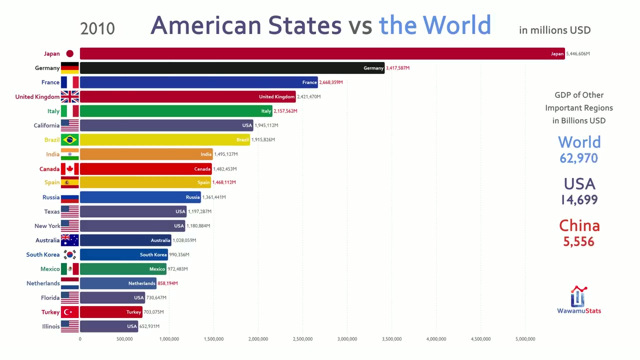 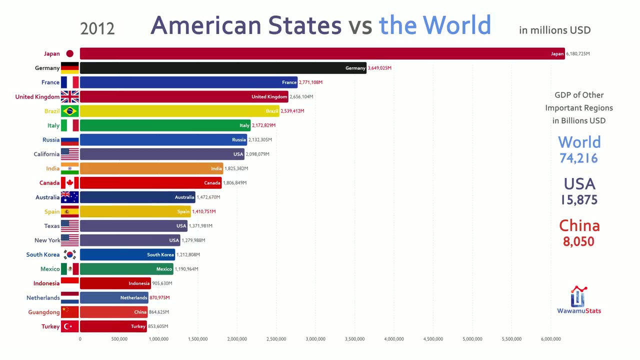 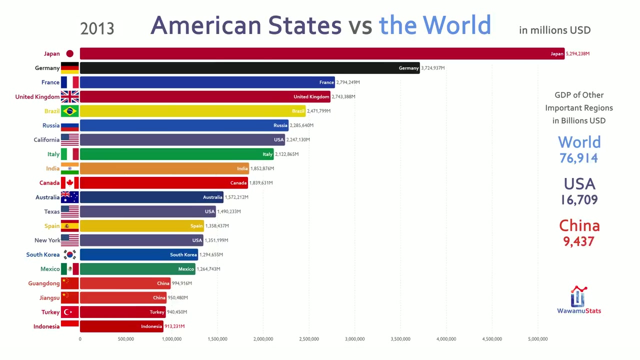 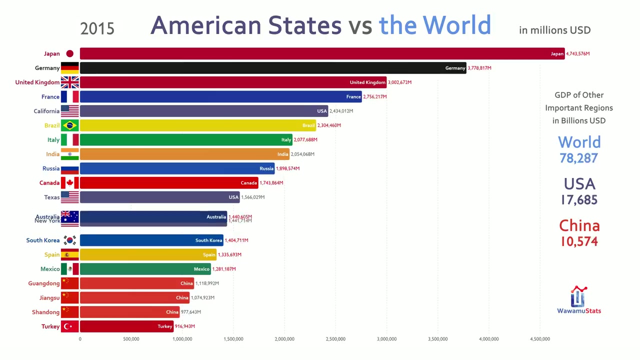 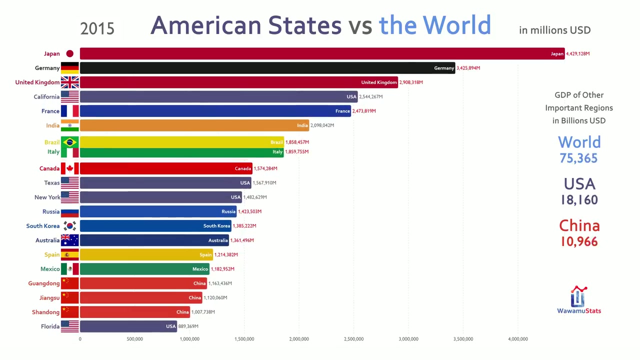 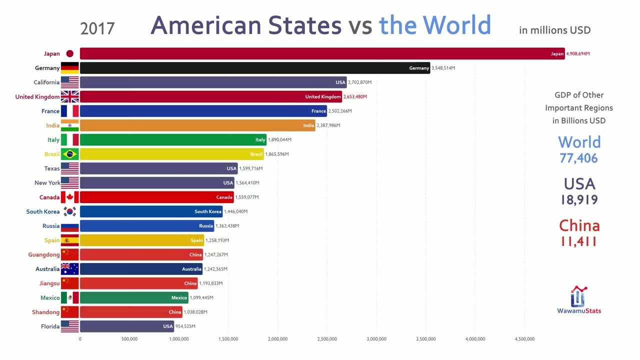 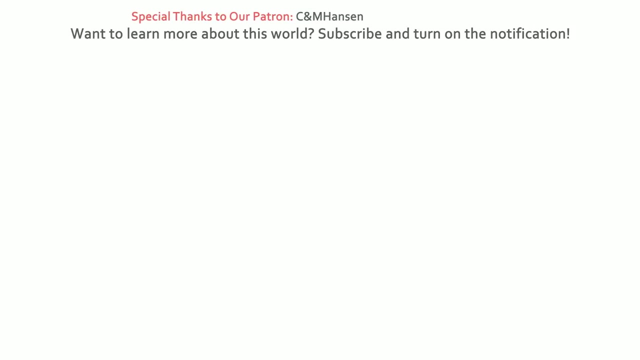